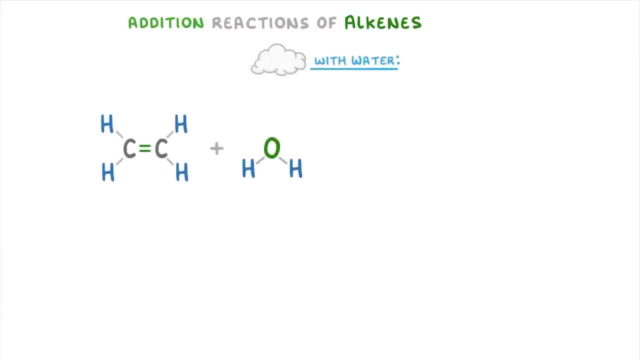 Next up, we have the reaction of an alkene with water, And this time we have ethene as our alkene. The conditions for this reaction are the presence of a catalyst and high temperatures, so that our water will actually be in the form of water vapour or steam. 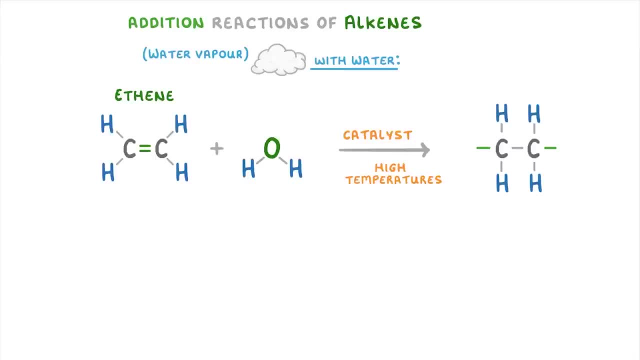 When they react, the double bond on the alkene opens up again and the water molecule will split into a hydrogen atom and an OH group. So this is a double bond reaction. So this is a double bond reaction which can then both go and bond to those carbon. 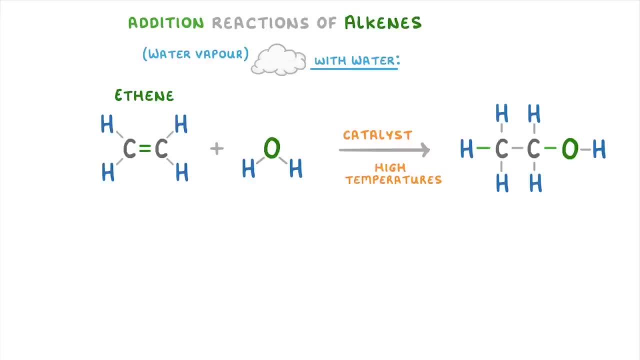 atoms. The product this time is called ethanol which, because it has this OH group, is a type of alcohol. And ethanol is actually the same alcohol as we use in alcoholic drinks and some industrial processes. This means that we do this reaction quite a lot in industry. 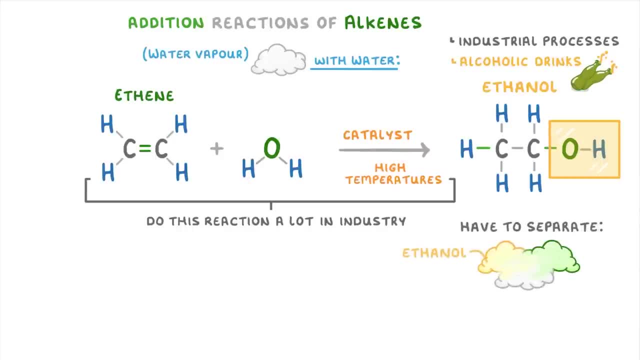 Once the reaction's taken place, though, we somehow have to separate each other out, and we'll have to separate the ethanol, which is what we want, from any unreacted ethene and water. The ethene is easy to separate because it has a relatively low boiling point. 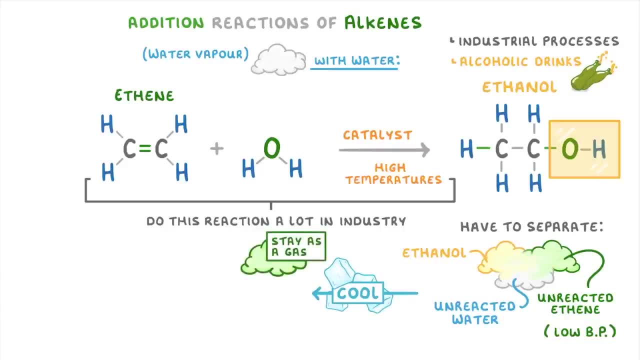 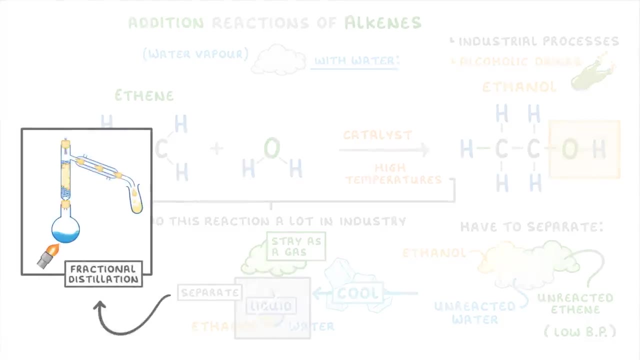 And so, if we cool down the mixture, the ethene will stay as a gas, while the water and ethanol will condense into liquid form. To separate the water and ethanol, though, we need to use fractional distillation. If you remember from one of our much earlier videos, this works by taking the mixture of: 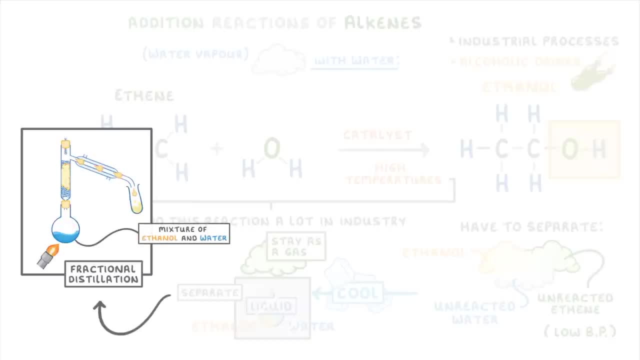 ethanol and water and placing it in a round bottomed heating flask. Then, as we heat it up, perhaps with a Bunsen burner, the ethanol will boil first, because it has a slightly lower boiling point than water does, And so it will evaporate up through the fractionating column and then condense into a separate beaker. 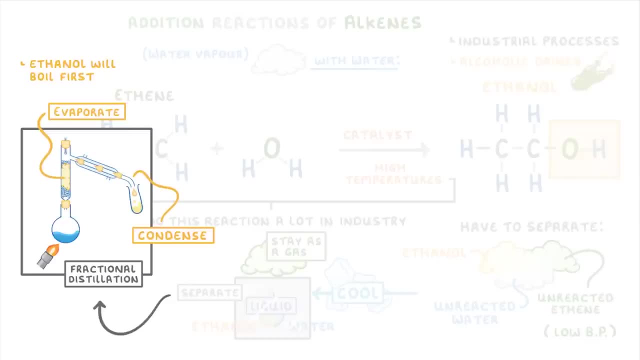 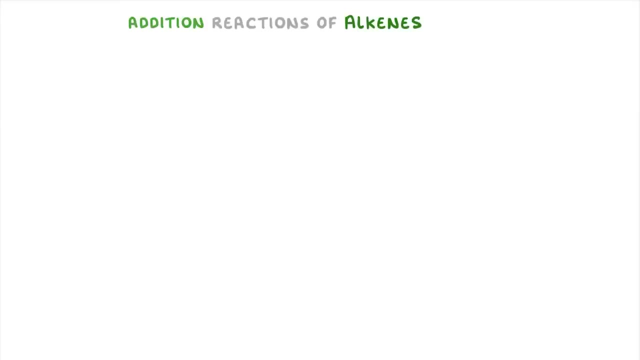 Whereas our water will remain in the heating flask because it didn't evaporate. The last example we need to cover is the reaction of alkenes with halogens. This is basically the same as the reaction with hydrogen that we saw earlier, But, importantly, it doesn't require any catalyst.